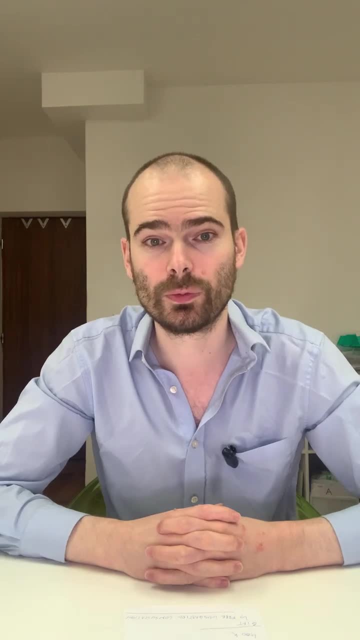 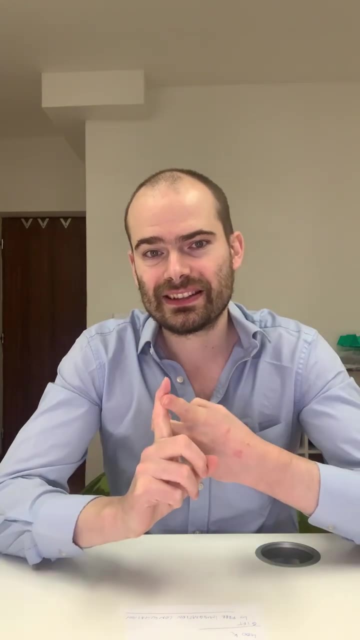 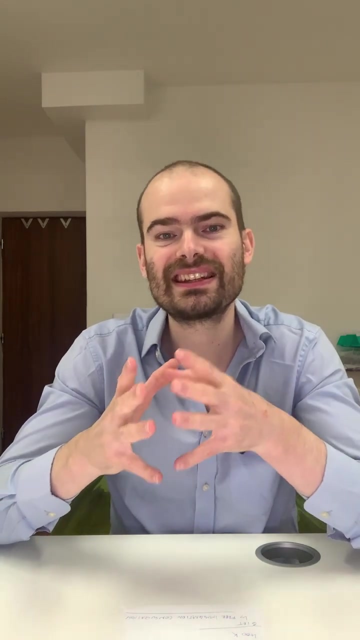 like, stabilize a bit and we will know what to expect from what companies. But as of now, the change, the prices change quite a lot. Second thing is that it that the price also depends on your status, If you're a student, and every company has a different definition of the student. In some, 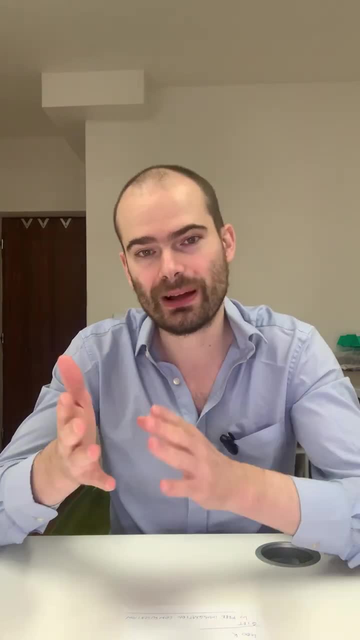 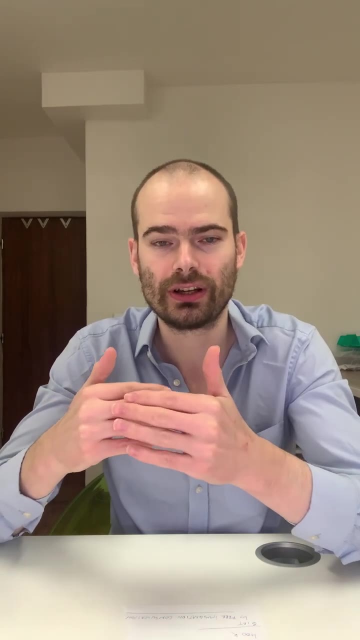 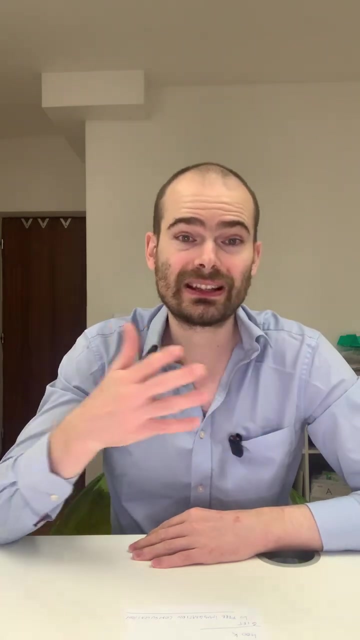 companies you have to provide confirmation of study. for some companies it's not important. Uh, for most companies the age is important. So for most companies the age uh limit is 30. So even if you study but you're over 30, you're no longer considered a student. Different companies: 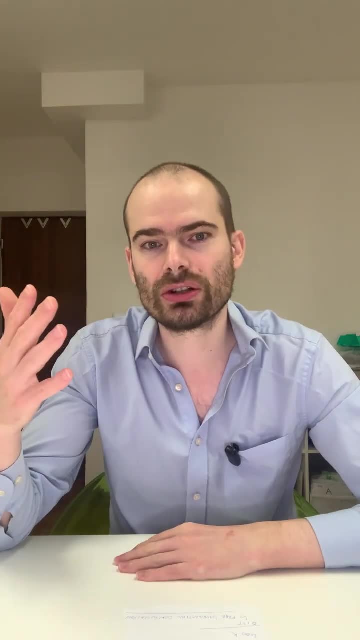 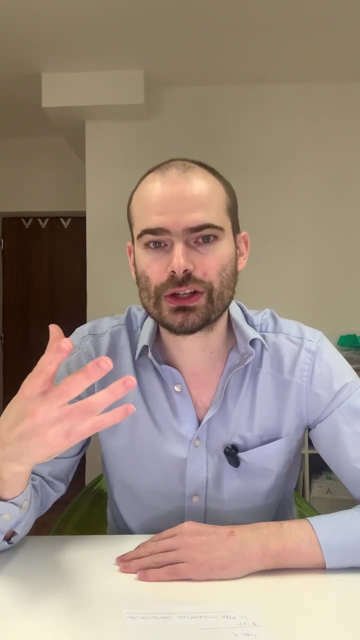 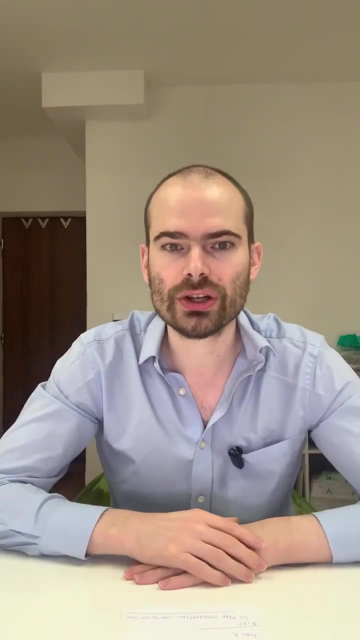 have different rules for that. And also, if you have some special requirements, like you're a pregnant lady or you need, like, a coverage for a professional sports or something, there are different- uh, different- pricings for that, so i cannot really share a price like that. but, as i mentioned, uh, if you get in, 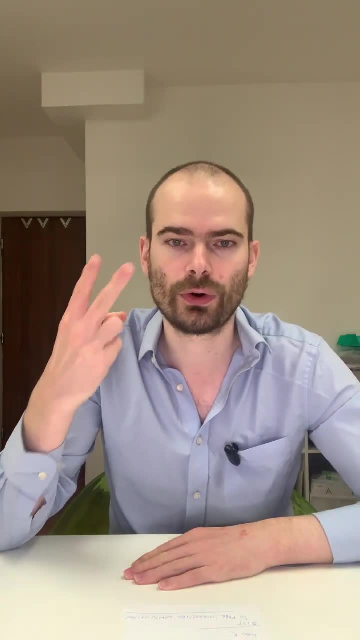 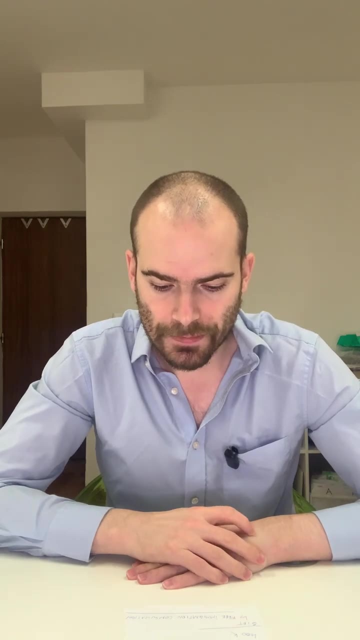 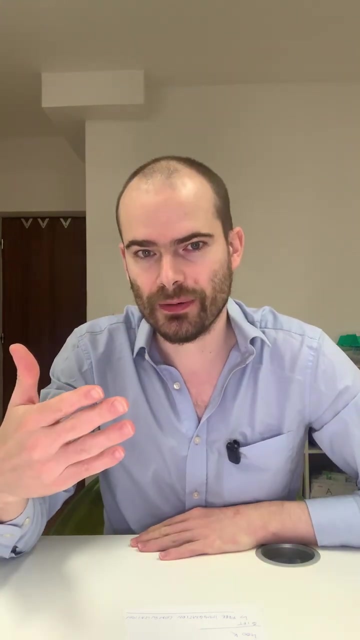 touch with the date of birth, uh, the type of visa you're applying for and the duration. i'll be happy to send you quotes from all the companies we work with. um couple confusions, or one main confusion, is that if you go pick up your visa, the embassy sends, and especially some embassies can send very confusing emails like: for the first three months you can get an emergency care and then after that you can. you, you have to get the comprehensive and then the the emergency must have that and that. so it's kind of weird from embassies that they do that, but yeah, that that's what happening. so, as of now most embassies will accept the emergency care for the first three months of your stay but the coverage must be at least four hundred thousand pounds, which i am not aware of any insurance company that would do that. they all have to do the 400 000 limit for the comprehensive because that became part of the new law canceling the monopoly. there is also this requirement that they had to increase the insurance limits to at least uh 400 000 euros, 10 million czech crowns. so all the insurance companies have the same coverage, uh, or higher than 400 000 euros. but that's for the, for the comprehensive. care for the emergency. i'm not aware of any insurance company that would offer that. i've tried three or four and none of them had it. uh, maybe the other two or other three have it, but generally no. so even if you wanted to get the emergency for the three months, the the embassies will not accept the insurance unless it has this coverage and none of them really has it. so you anyway should get the comprehensive, comprehensive for the full validity of your stay and anyway it makes most sense like the only advantage of getting the three months of. emergency would be the price, because the emergency is significantly cheaper than the comprehensive. on the other hand, the coverage is also significantly lower. so if you get three months of, uh, emergency care and something happens within the three months, yeah sorry, you only have emergency care so, but you didn't pay much for that. so anyway, from this perspective, i would recommend getting the comprehensive anyway. plus, it will be way easier for you because you will be buying a comprehensive from or like the emergency, for three months from one company and, like you, will have one contract and you have to make one payment. then you will. 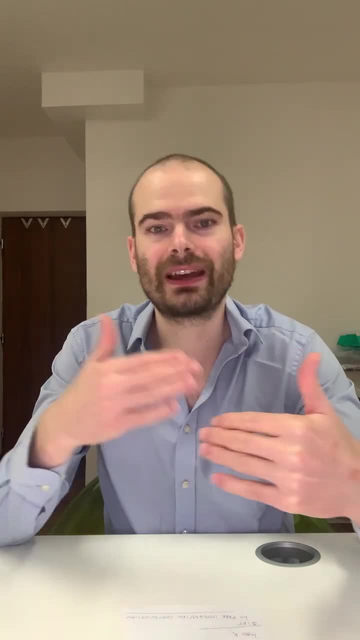 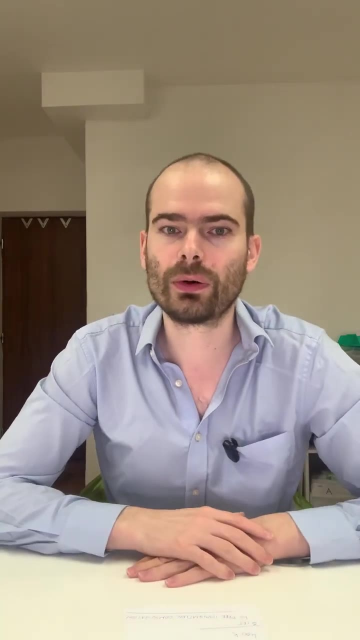 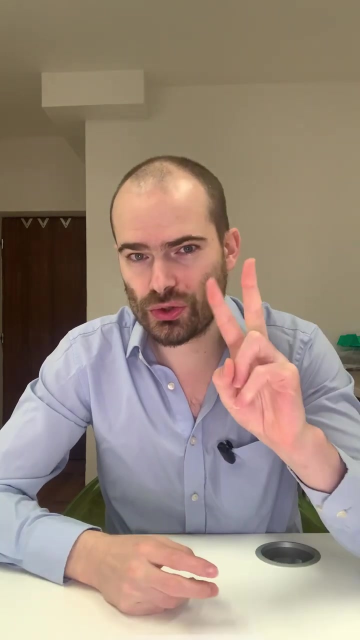 be getting the comprehensive from another company and you will have another contract and you have to pay again. so you'll have two companies, two insurance contracts, two cards, and it will be only confusing, plus the coverage will be anyway. so one thing, uh two, two more like things, one, and i will get to the gift in like one minute. this is. 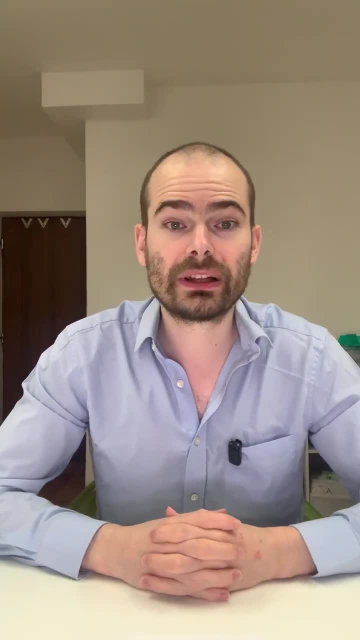 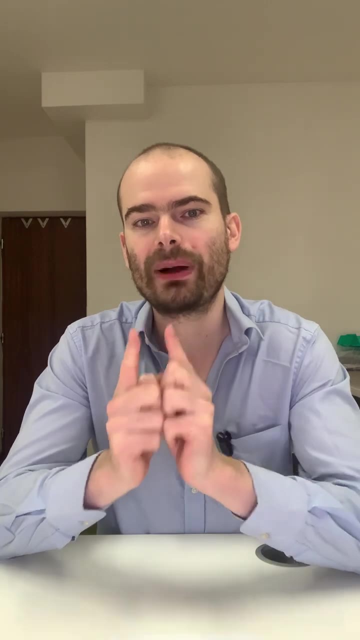 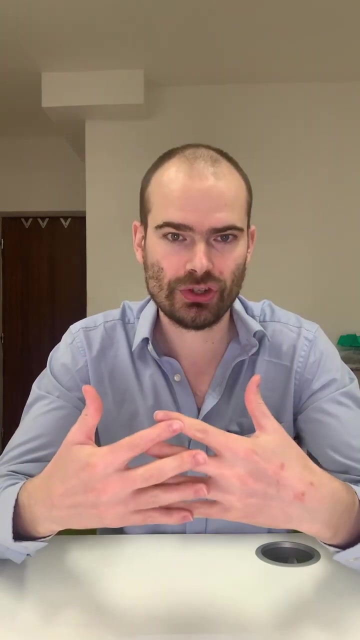 just one thing i want to say: uh, and then i will. i will give you the the surprise gift which we have for you. so there is a difference between the embassy and the moi. the general difference is that for applications submitted at the embassy- czech embassy- or in the country of your origin. 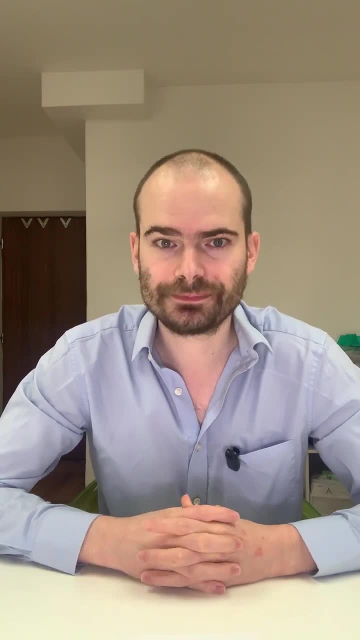 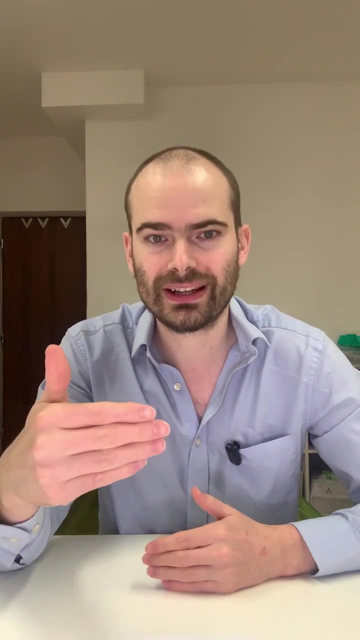 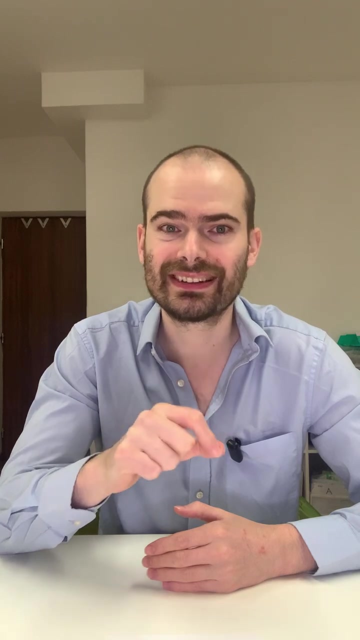 or somewhere else. you don't need generally to submit the insurance when you're submitting the application. you have to have the insurance only once you go collect the approved visa at the ministry of the interior. it's the other way around. you have to, in most cases, submit your insurance when you're submitting your application. so that's the main. 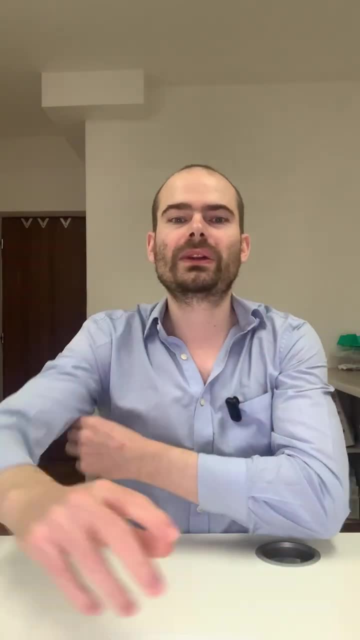 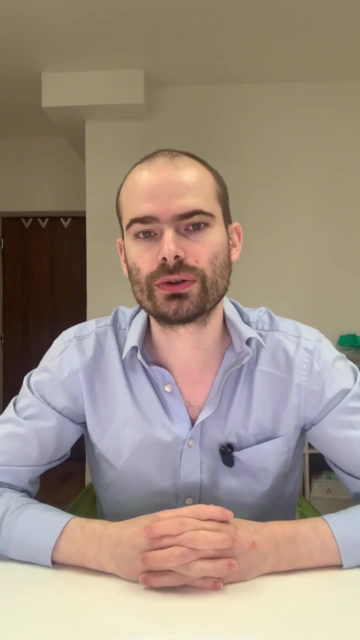 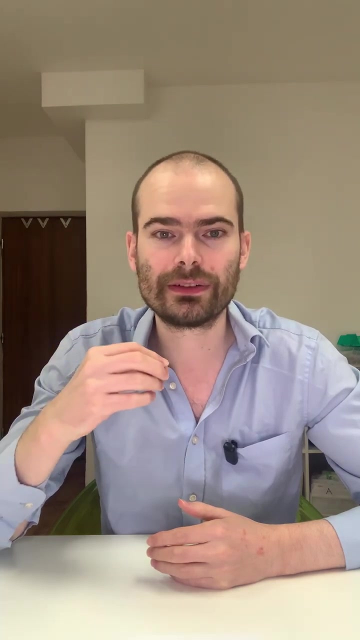 difference. and now the, the gift i promised, what we decided to do, uh, in move to prague as a, as a support for you- is that when you get insurance from us- and that doesn't mean that it will be more expensive, it actually might be even cheaper than what you can get online or through. 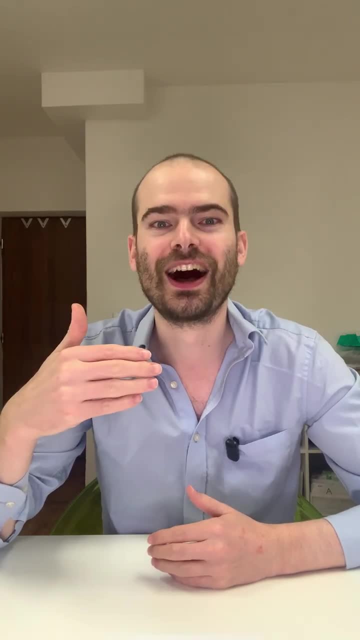 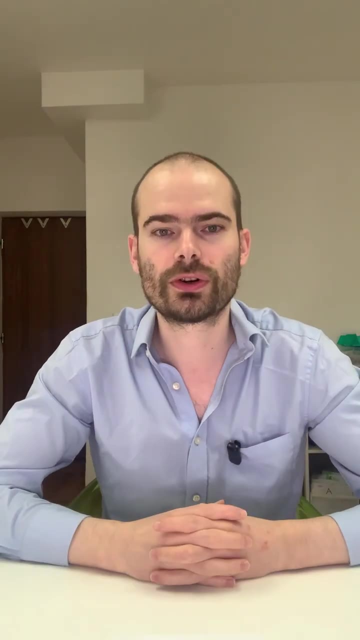 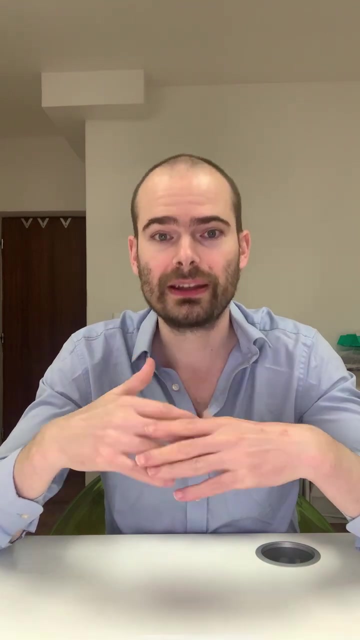 some other vendors, because we've done a lot of insurance for all the insurance companies so we generally have the lowest prices you can get. plus we don't charge, of course, any commission on that. so whatever you, whatever, we calculate in the system of the of the insurance company you're. 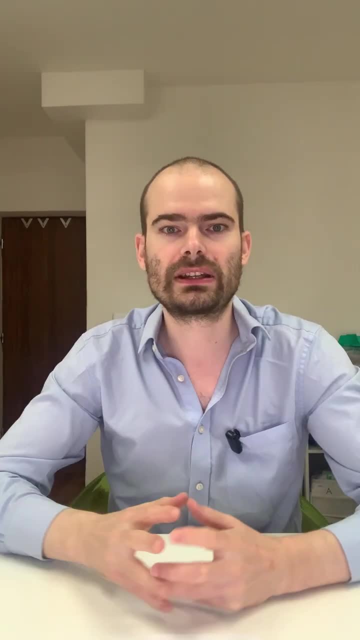 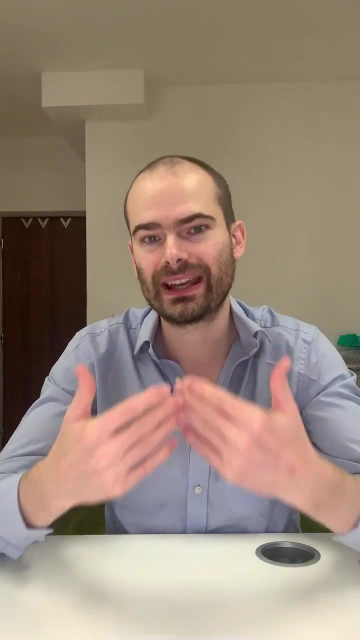 doing with that trained, so there has to be the subservient to get that. cons cuerpo and uh came up with the accounts addicted, right, but the thing, what we have here is that if you go to the insurance company, you will get, and it's basically everything. 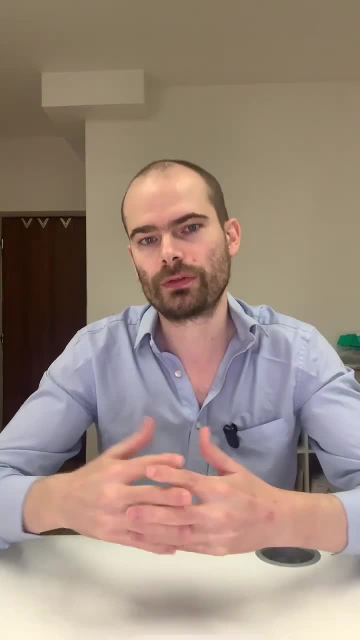 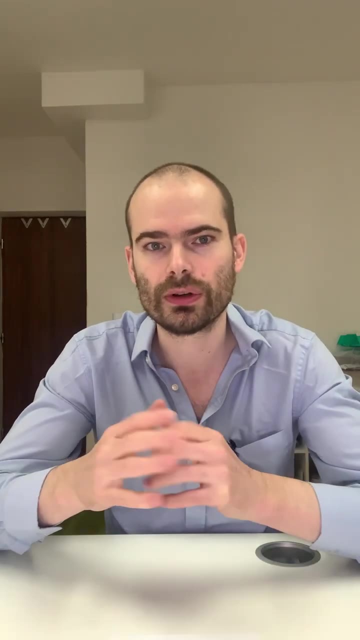 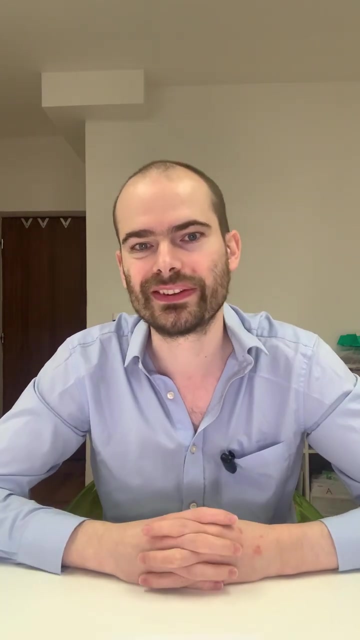 going to the uh, to the insurance company, so you will have the lowest possible rates. and also, if you get the insurance through us, then we will give you a free immigration consultancy on top of the insurance. so you come to us for insurance, someone to visit, or if you just have any questions. you want to get a trade. 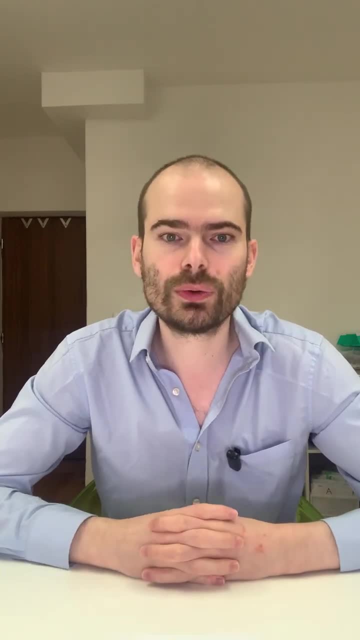 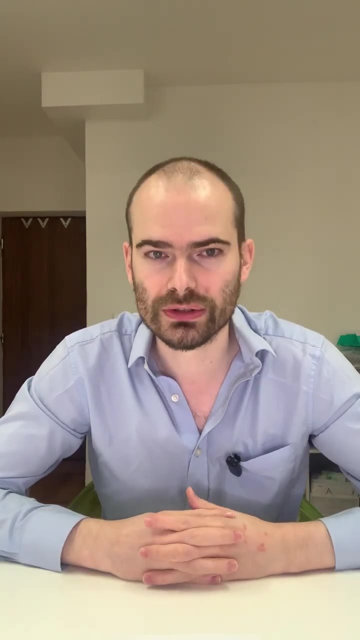 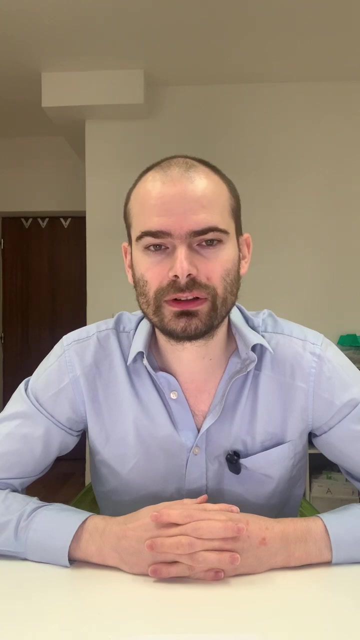 license in the Czech Republic. you want to find a flat or something, so you will get. with every insurance contract you will do with us, you will get a free immigration consultation. this will be valid until so far, until the middle of December. we'll see if we'll extend it until the end of December. maybe yes, but